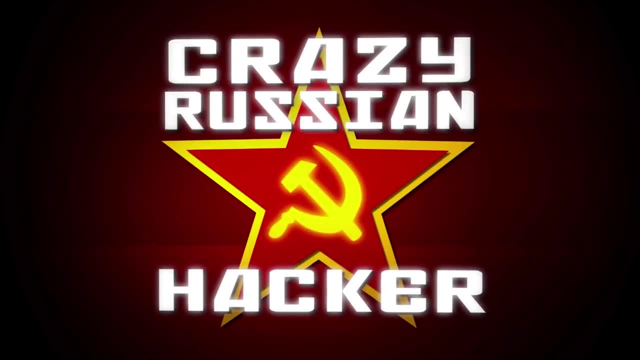 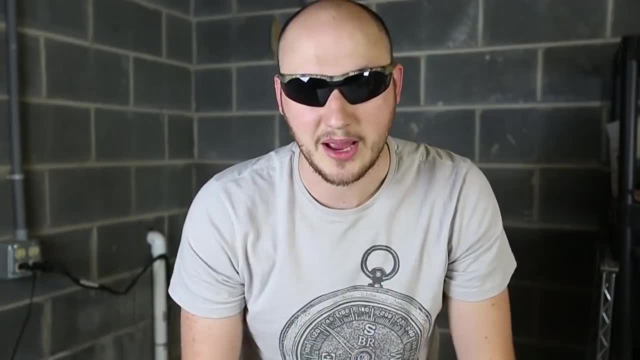 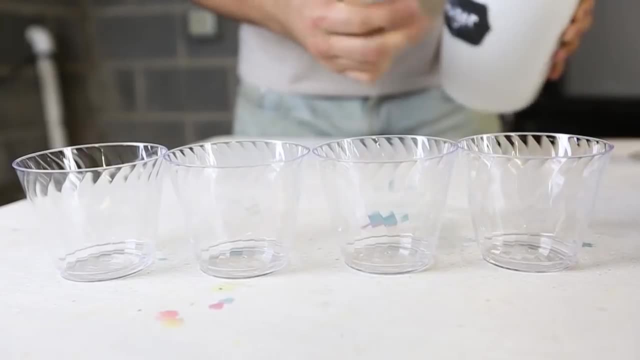 What's up everybody? welcome back to my laboratory, where safety is number one priority, And today I'm going to show you very easy but very cool sugar density experiment. Let's check this out First. we're gonna need four empty plastic cups, tablespoon and sugar. 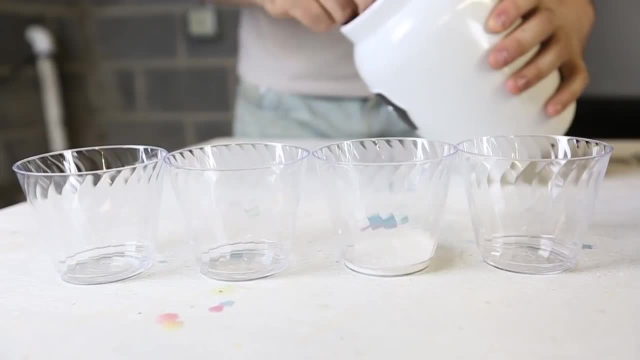 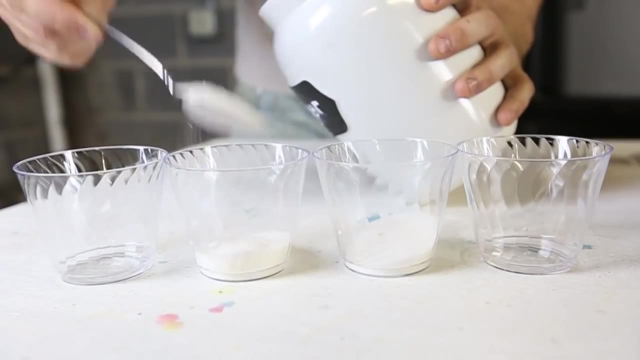 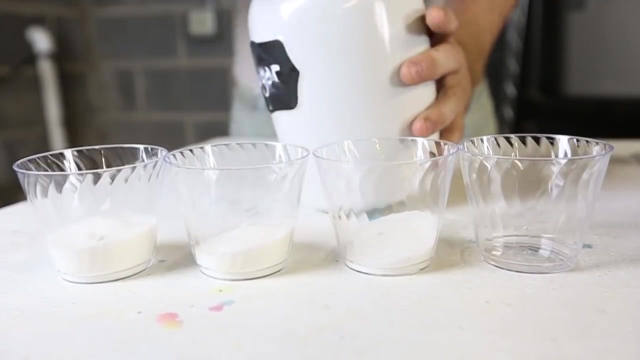 In first one we won't put any sugar. In second we're gonna put two tablespoons of sugar. In third one we're gonna put three of them, And in fourth we're gonna put four. Then we're going to put about sixty milliliter of water. 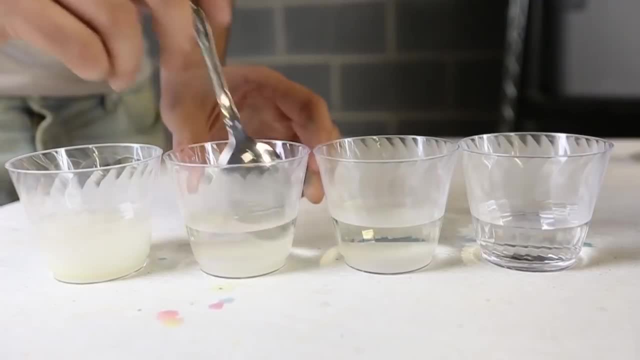 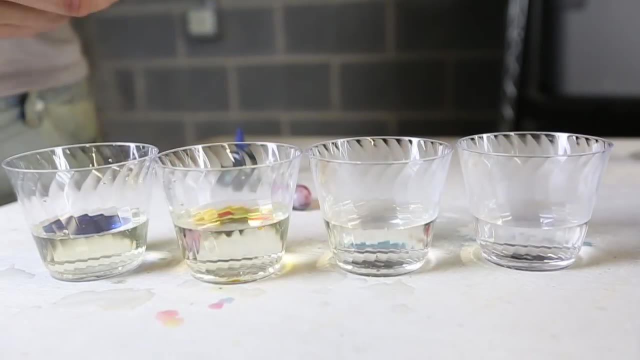 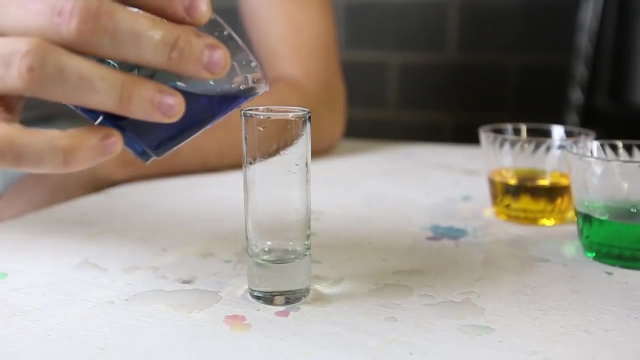 I'm using warm water so it will be easier to dissolve all the sugar. Then we're going to put food coloring, Mix it all up once again. Then we're going to grab blue water which has four tablespoons of sugar and pour it just like this. 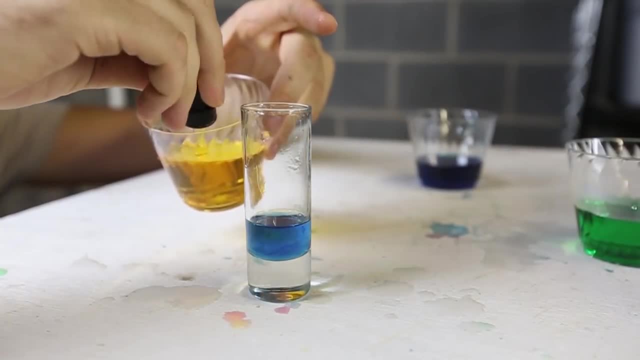 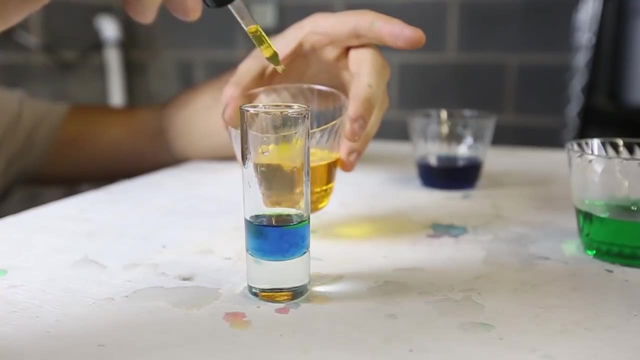 The next layer. we need to pour really, really slowly. So I'm gonna grab a syringe or something and just stack all that water right on top of this other water. You don't want to mix it up, so you want to pour it very slowly. 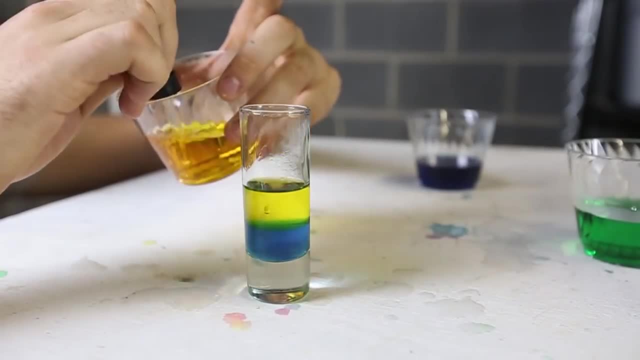 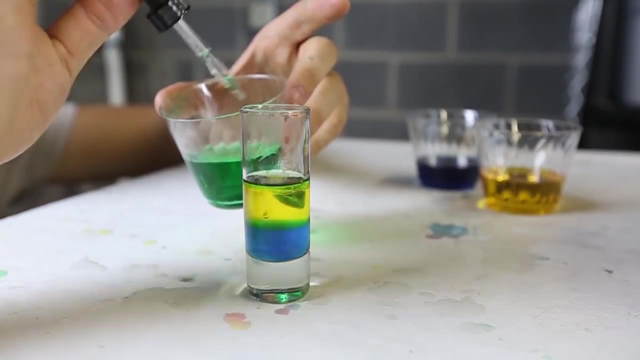 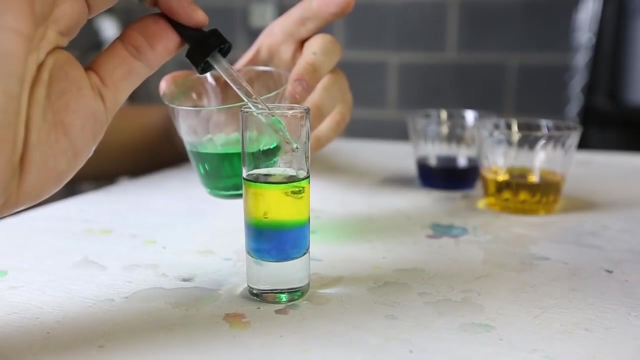 As you can see, we have two layers now: Blue and yellow. I wish I had a bigger syringe. that way I can fill it up much, much faster. But yeah, use the rim of the glass to pour the liquid down. Look at how beautiful it is. 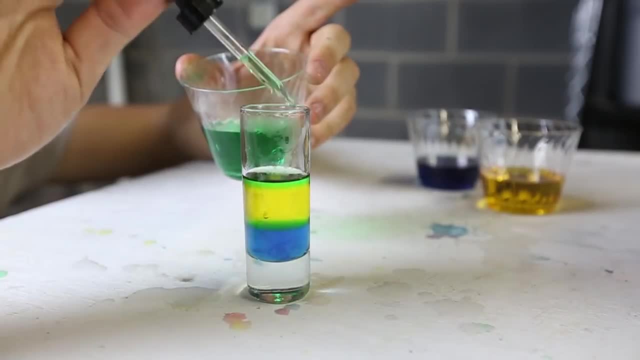 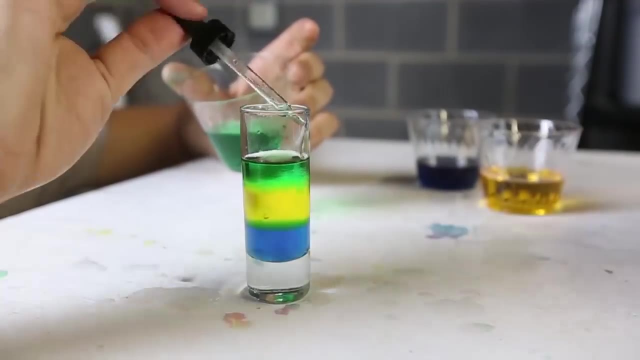 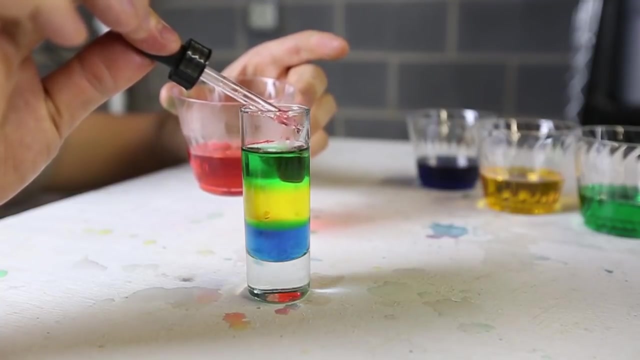 You see how it's stacking up already. And then the last one, the red one, doesn't have any sugar at all. Again, gonna pour it very slowly because I don't want to mix them. You see the red one starting to form.